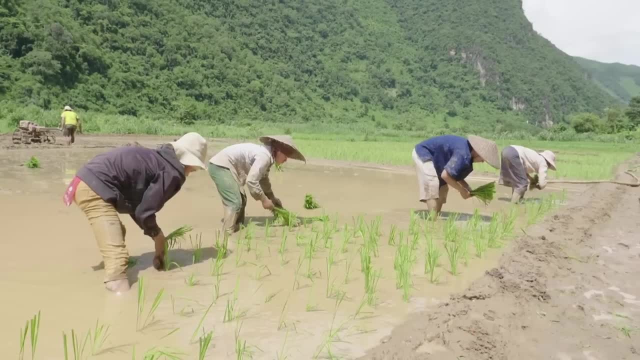 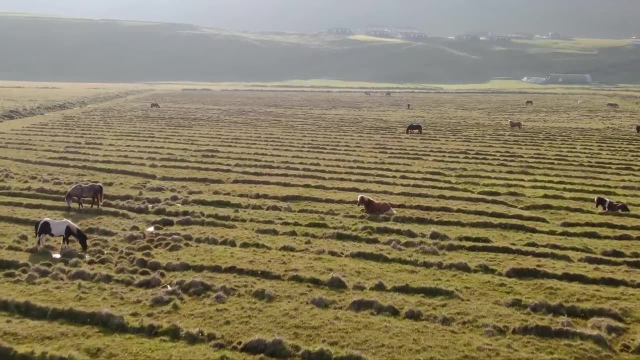 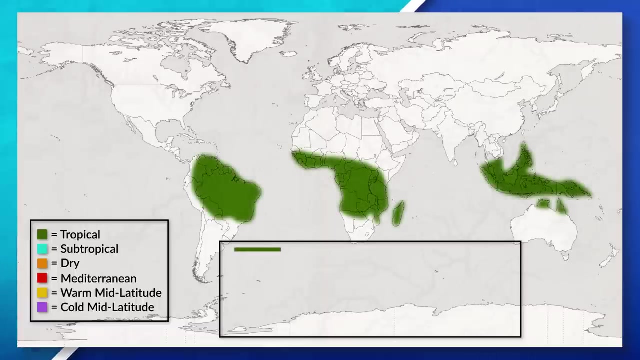 hear different languages and dialects, see different types of agriculture and, most importantly, try different food. Oftentimes we can see different agricultural products grown and produced in areas with specific physical environments. We could look at tropical climates, such as in Indonesia or countries in Africa near the equator, where we'll see the production of coffee, sugar or pineapple. 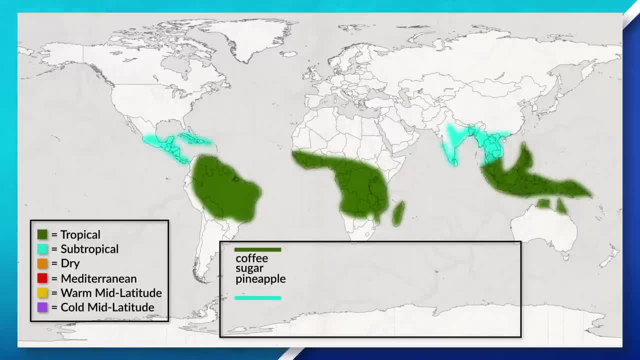 If we look at subtropical climates such as the West Indies or parts of Indonesia, we'll often see rice, cotton or tobacco In the grasslands and continental steppe that contain areas such as Mongolia, the western portion of the United States. 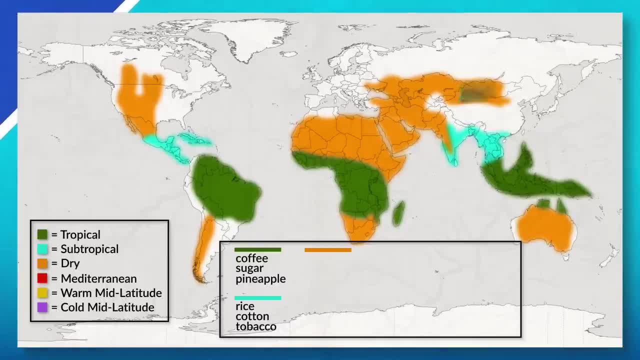 or states located in northern Africa, we often see cattle ranching sheep, goats, horses or camels, While Mediterranean climates, such as California, Chile or geographic areas that surround the Mediterranean Sea, will often see the production of grapes, olives and dates. 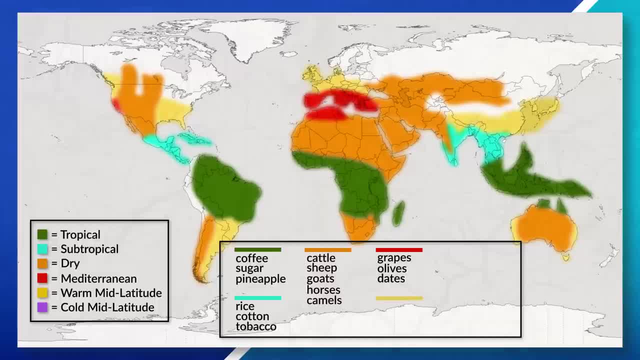 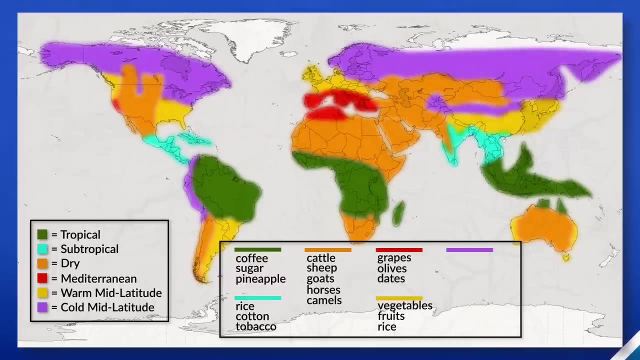 Moving into warm mid-latitude climates like southern China and southern parts of the United States, we often see different vegetables, fruits and rice being produced. Lastly, we have cold mid-latitude climates such as the north-central part of the United States, southern Canada and eastern Europe. 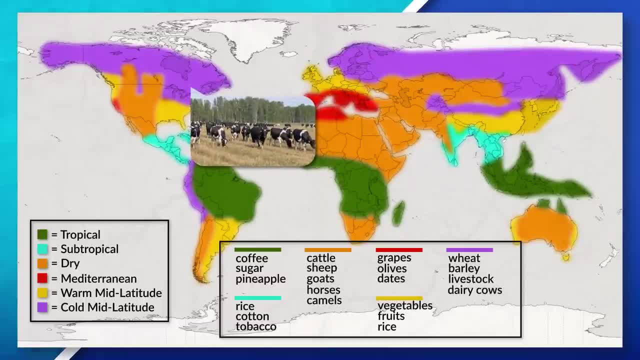 where wheat, barley livestock and dairy cows are often grown and produced. Notice that each of these different climates leads to the production of different foods. This is due to the distinct physical features of an area and the climate. Some of these areas offer longer growing seasons. others have more arable land. 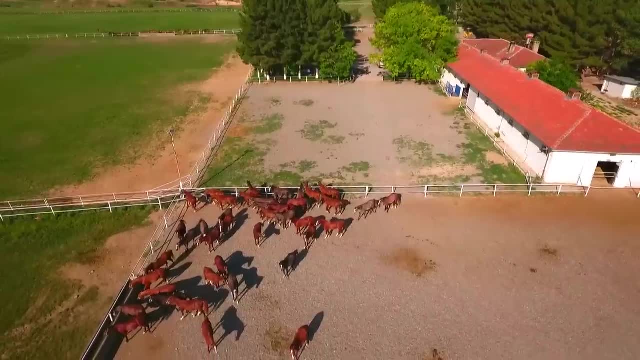 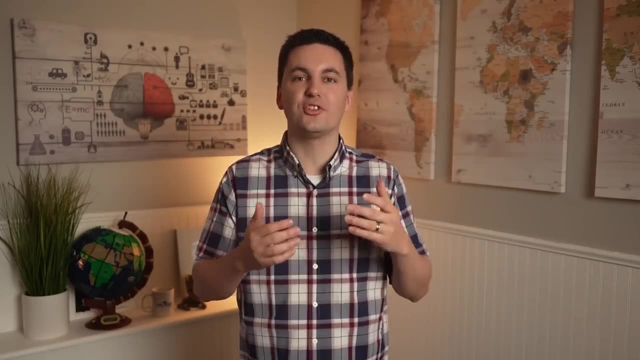 some have more access to fresh water and others have more space for the production of different agricultural goods. Today, the barriers to growing food are steadily being reduced thanks to advancements in technology. Farmers today can use different fertilizers, herbicides and pesticides. 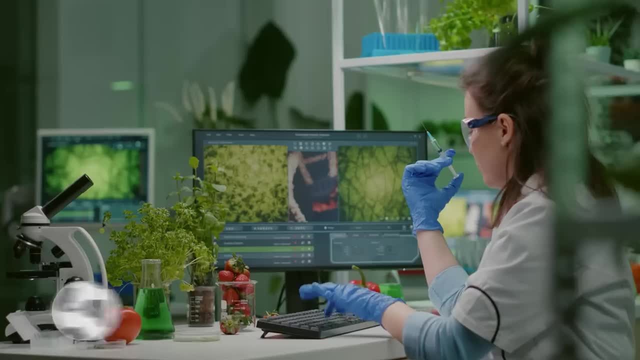 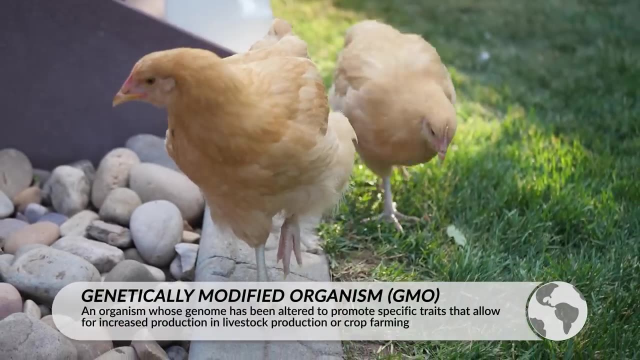 to increase the yield of their crops. Genetic modification of plants and animals has also allowed for crops and animals to grow faster and larger and environments that they used to not be able to grow in New methods of farming, such as greenhouses, vertical farming and community gardens and farms. 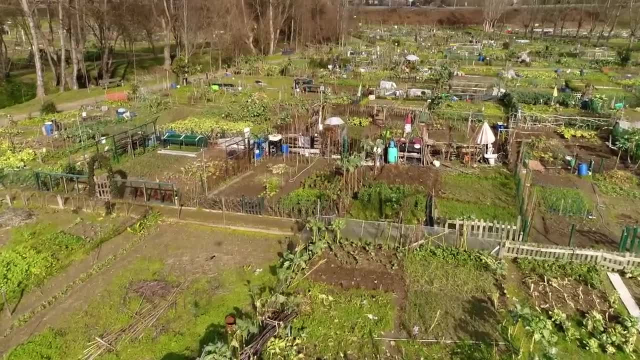 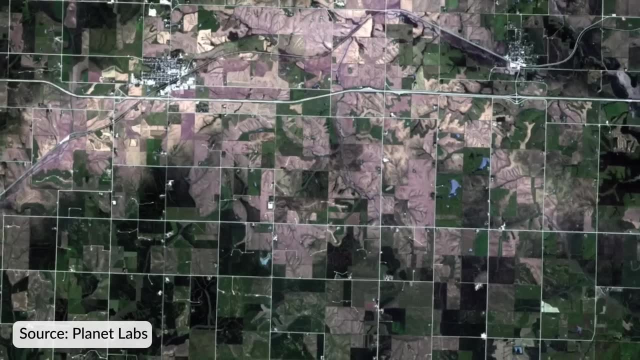 allow for food to be produced in and near urban areas on land that used to not be able to grow. Plus, that's not even mentioning advancements in irrigation, GPS and GIS, which allow farmers to better understand their crops when they need water fertilizer. 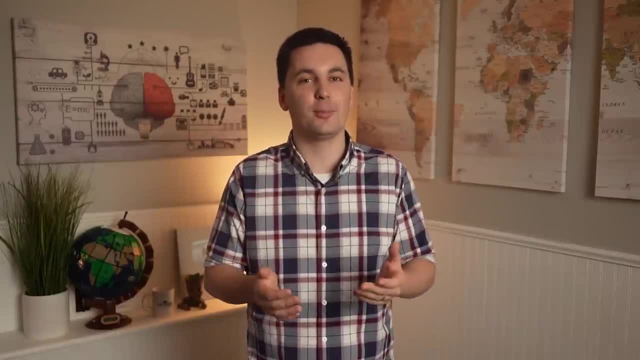 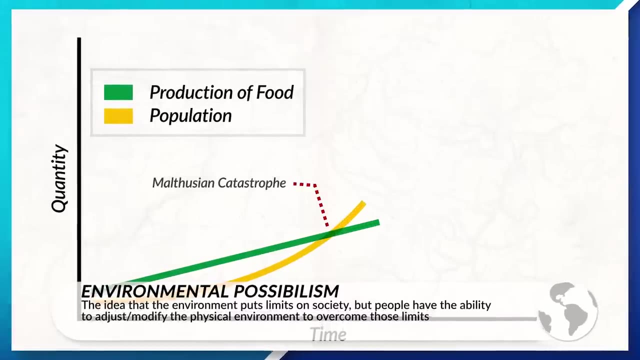 or when they're ready for harvest. All of these advancements are great examples of environmental possible-ism, a concept we last talked about in Unit 1.. And all of these advances counter Thomas Malthus' original idea that food production growth is arithmetic. 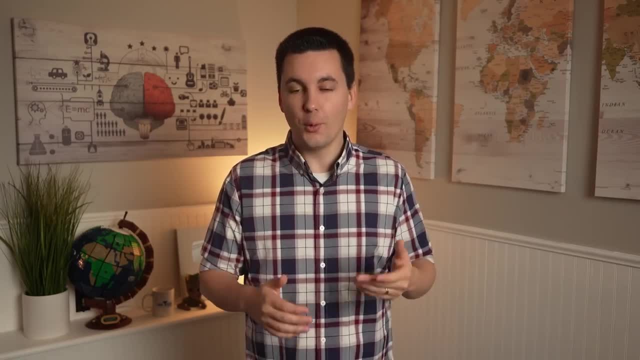 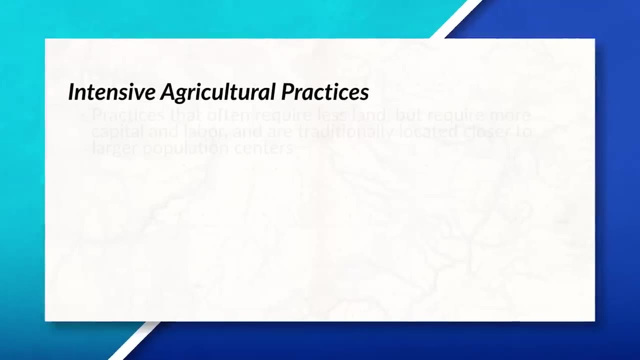 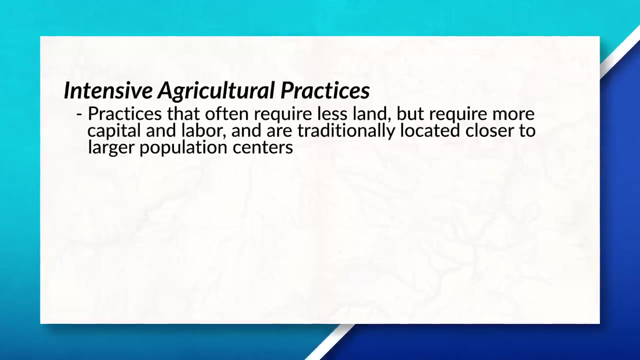 Now, when looking at different types of agriculture around the world, we can see different types of intensive practices and extensive practices. Intensive agricultural practices often require less land, but require more capital and labor. They're traditionally located closer to larger population centers. 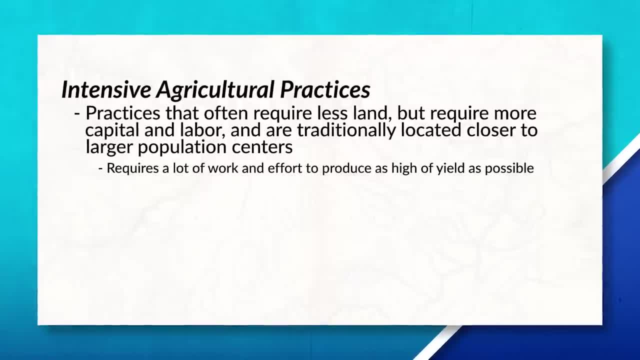 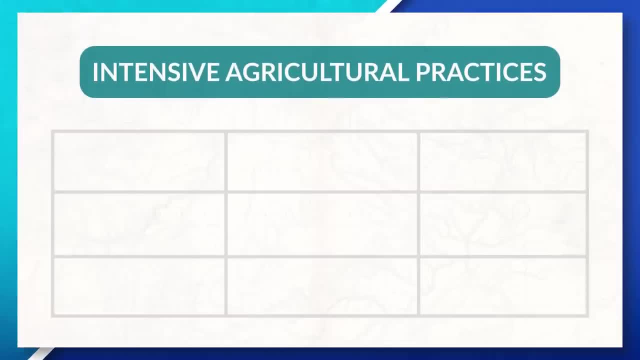 This type of agricultural production requires a lot of work and effort to produce as high of a yield as possible. Today we can see a variety of intensive agricultural practices around the world. Plantation agriculture is traditionally located in periphery countries and former colonies that are located in rural areas. 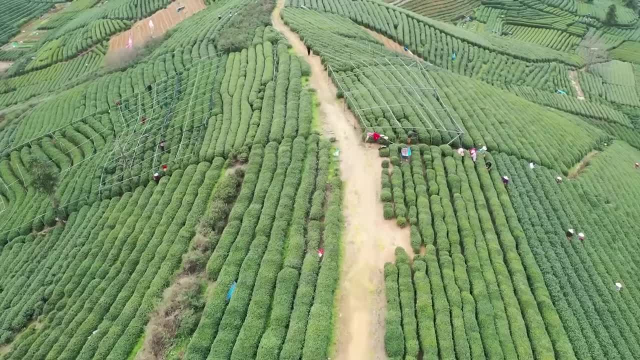 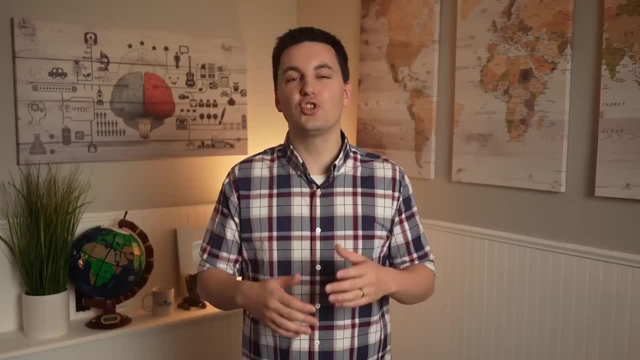 Plantation agriculture is traditionally located in tropical climates that have longer growing seasons. Labor in these areas is often cheap, which reduces the cost of production. We can see that many of the crops that are grown on plantations are cash crops, which are crops that are grown for the sale on the market and not used by the grown. 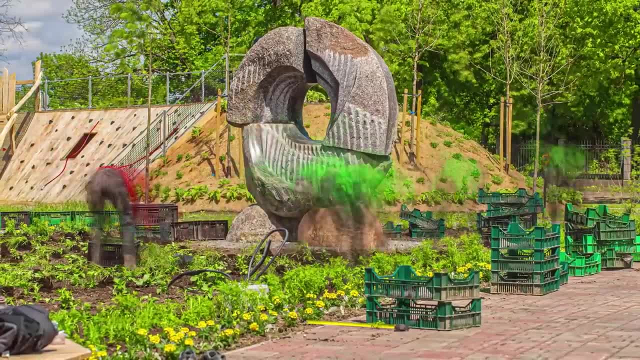 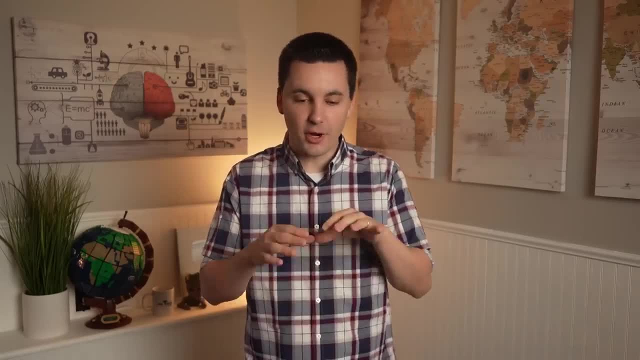 Oftentimes we may see farmers in areas that have less economic development grow cash crops to export their crops to more advanced economies to generate income, which can create issues for developing countries. Farmers are often forced to export food instead of produce food for their own people. 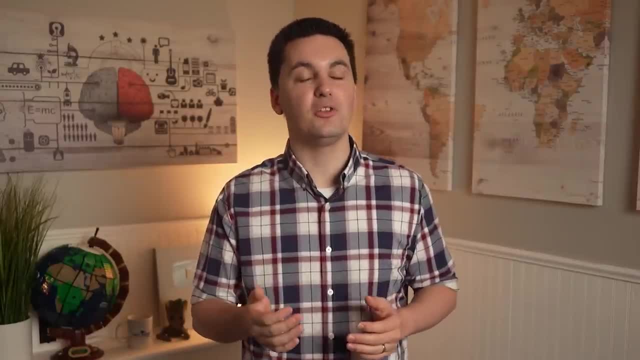 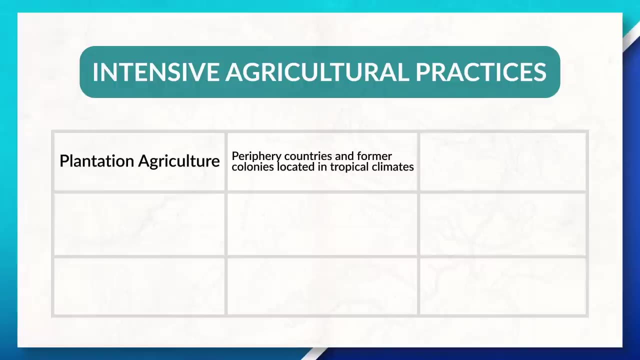 Today, many of the plantations around the world are run and operated by companies in more economically advanced countries, with the goal of exporting the food produced in the plantation to core countries. Plantations often grow either coffee, sugar, tobacco or tea, just to name a few examples. 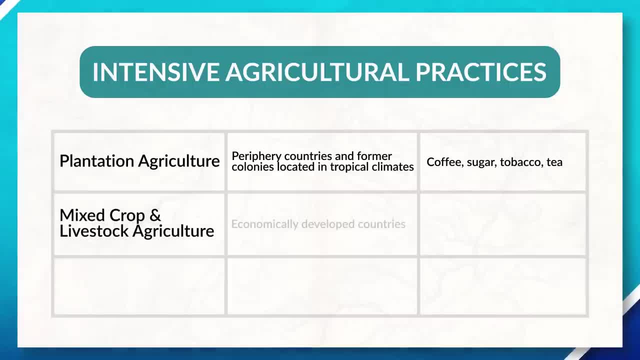 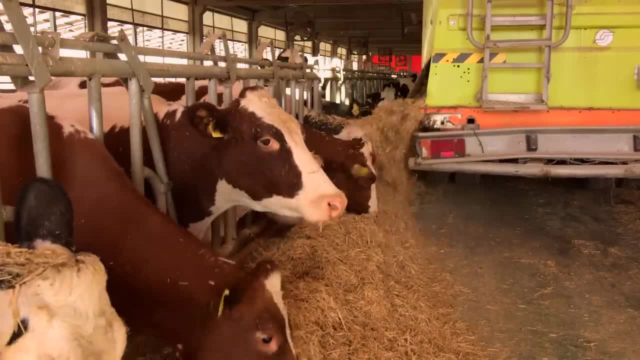 The next intensive practice is mixed crop and livestock agriculture, which is typically found in more economically developed countries. These crops are often used to feed and fatten the livestock. Once the livestock is ready for sale, it will be sent to the slaughterhouse processed. 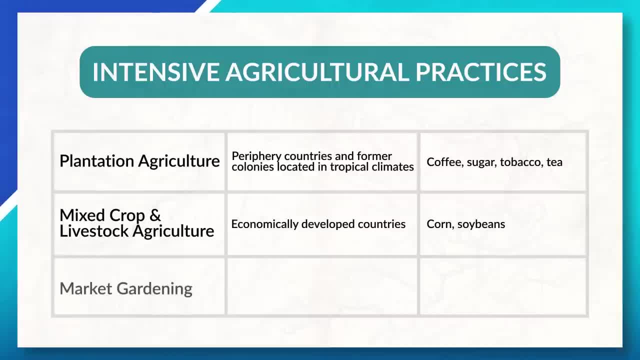 and eventually sent to the market for sale. Lastly, there is market gardening, also known as truck farming. This is located in geographic areas that have longer growing seasons, such as the southeastern part of the United States. Here, farms often grow fresh fruits and vegetables. 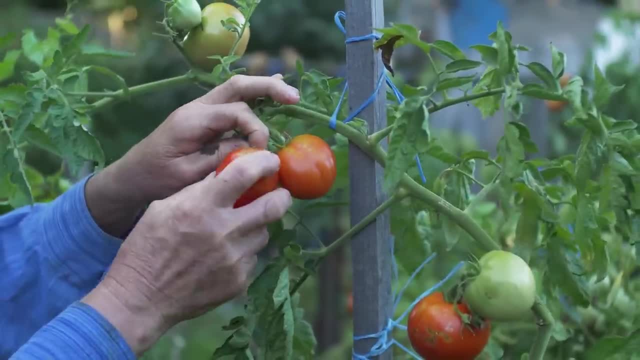 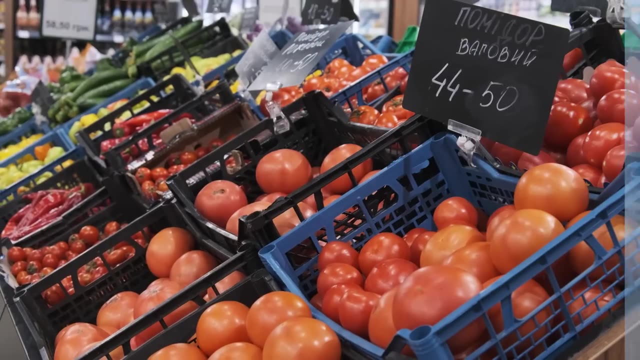 The food is often harvested by migrant labor to help keep costs down, and once picked, it's either frozen, canned or frozen. Then it's put onto a truck and shipped out to the market, where it will eventually be sold Now. extensive agricultural practices, on the other hand, tend to use less labor and 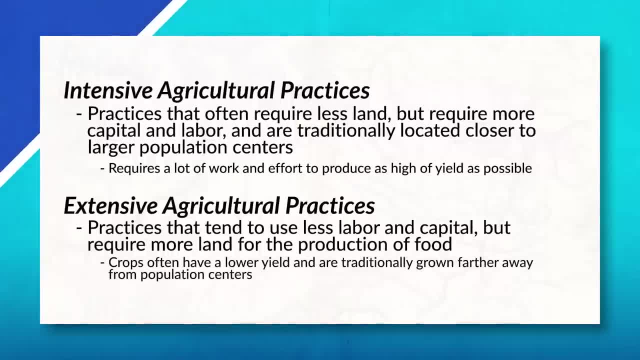 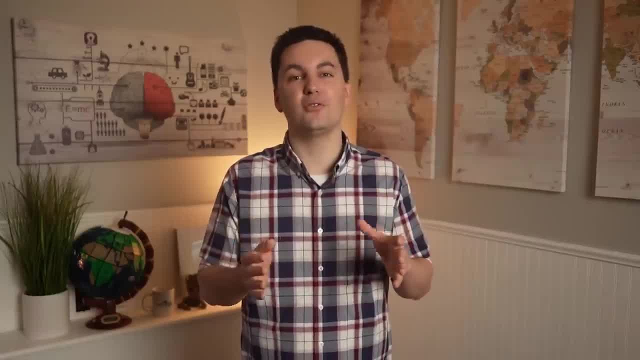 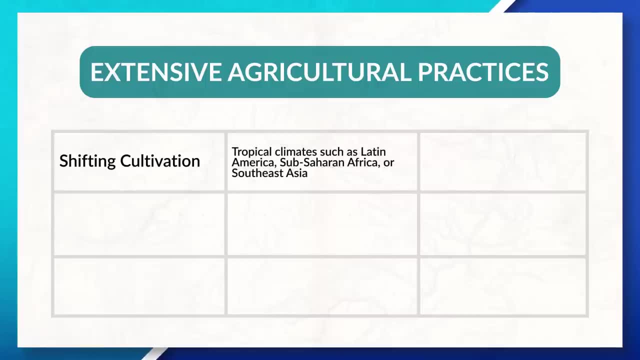 capital, but do require more land for the production of food. Crops often have a lower yield and are traditionally grown farther away from population centers. Today, we can see a variety of extensive agricultural practices around the world. Shifting cultivation is often located in tropical climates such as Latin America, sub-Saharan. 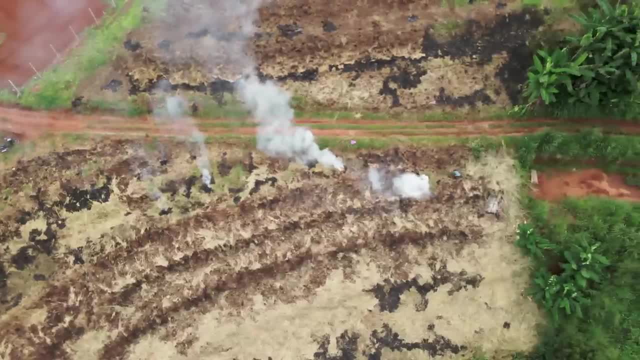 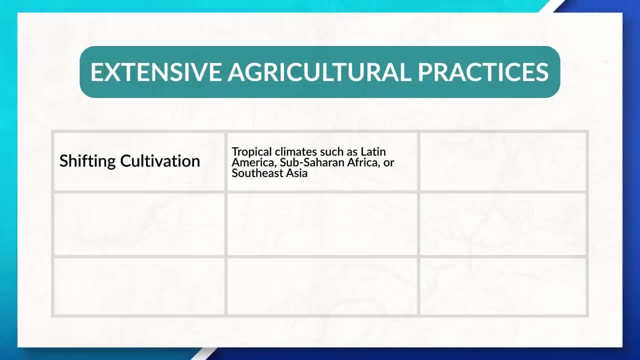 Africa or South Africa. This type of agriculture involves finding a plot of land, typically in a rain forest, and designating it for agricultural use. The land will then be cleared and crops will be planted continuously in the clearing until the land starts to become less productive due to a loss of nutrients in the land. 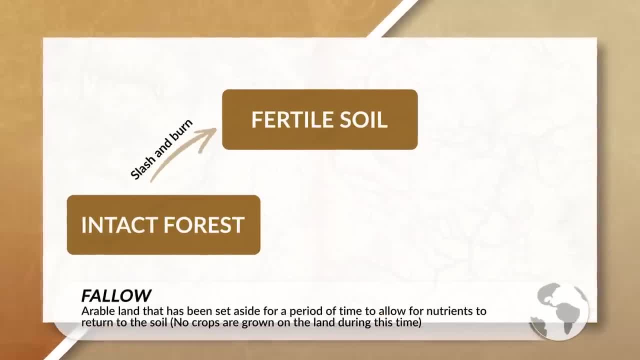 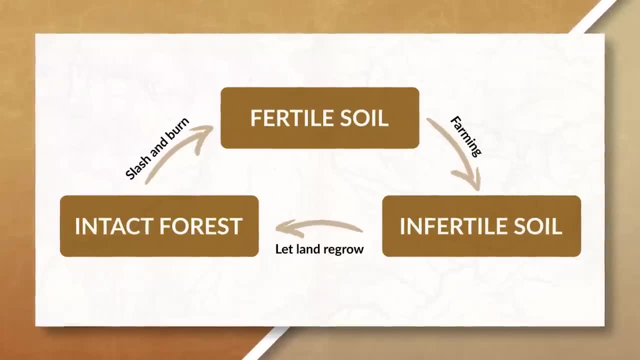 After that, the original plot of land is left to follow, which means the land will be left alone to allow for vegetation to regrow and nutrients to return to the soil. A new plot of land will then be identified and the process will repeat. 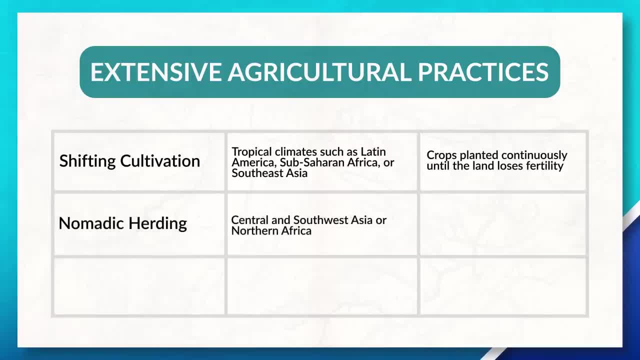 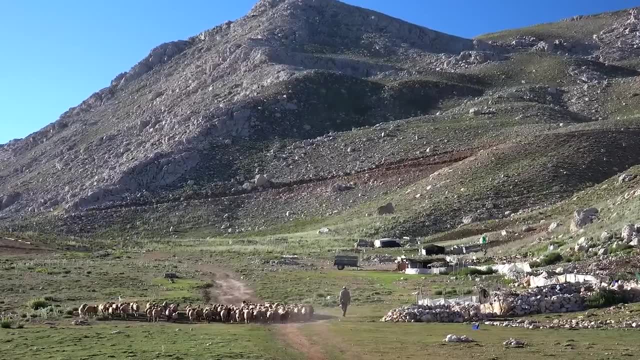 Moving over to agriculture, there are a number of different types of agriculture. Moving over to Central and Southwest Asia or Northern Africa. we can see nomadic herding Here. sedentary agricultural practices are not practiced because the physical environment does not allow for traditional farming to occur. 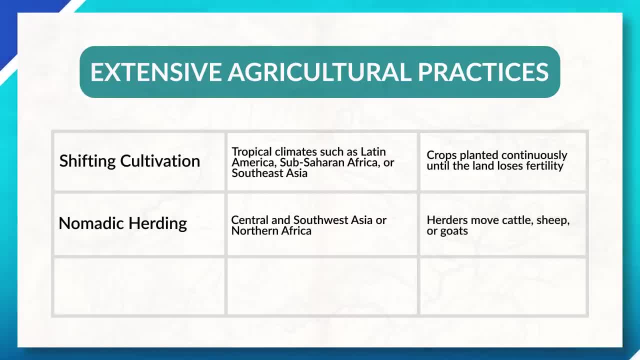 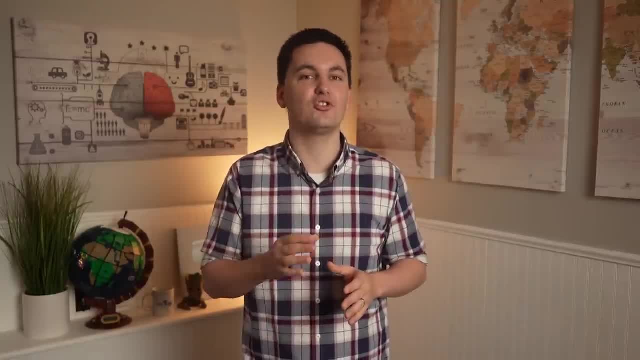 People. instead are herders who move with their animals, which are traditionally cattle, sheep or goats. Herders here are constantly on the move and are nomadic, but they tend to stay in a set geographic area. Oftentimes, due to the constant movement, the population size is limited and people 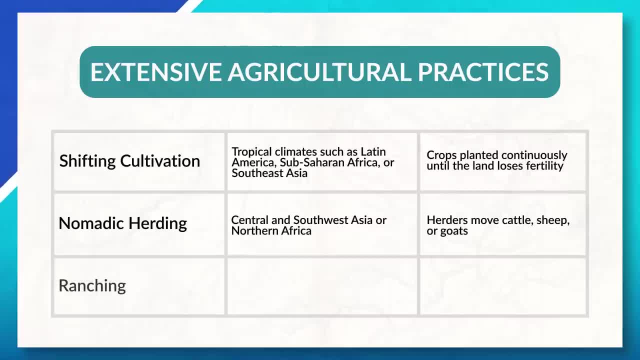 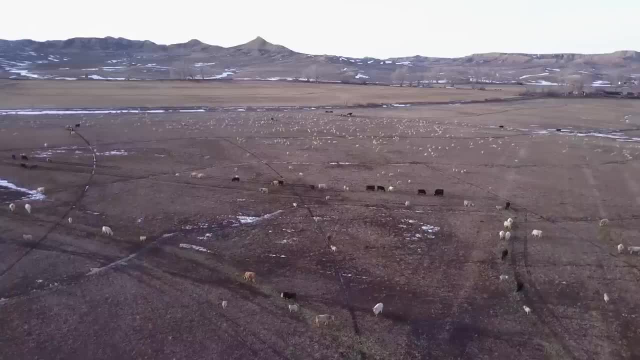 tend to possess few possessions. Lastly, there is ranching, which is typically located in areas where the land is not ideal for farming. This often means that land is less expensive, which is important since ranching takes up a lot of land. This type of extensive agriculture is also located farther away from population centers.